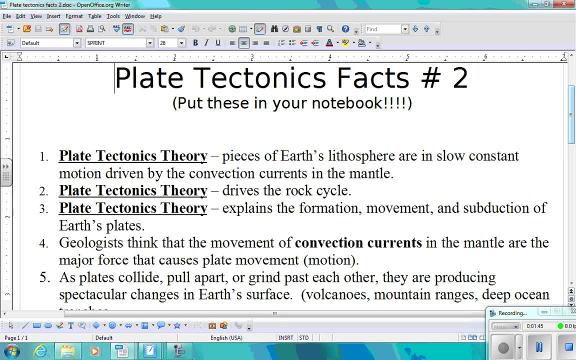 There are 10 facts here. I would like you to copy them into your notebook. Play tectonics theory. Pieces of earth's little lithosphere are in slow, constant motion, driven by the convection currents and the mantle. Play tectonics theory drives the rock cycle. 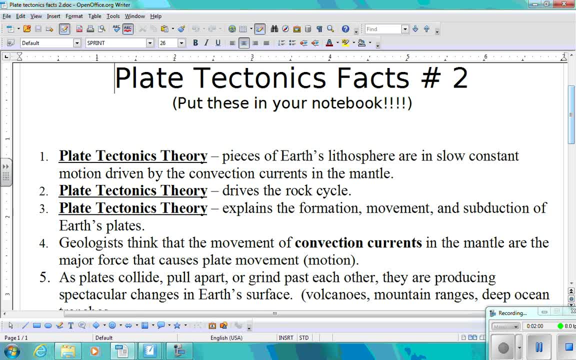 Play. tectonics theory explains the formation, movement and subduction of earth's plates. Geologists think that the movement of convection currents in the mantle are the major force that causes plate movement. And remember, that was what Alfred Wagner could not prove. 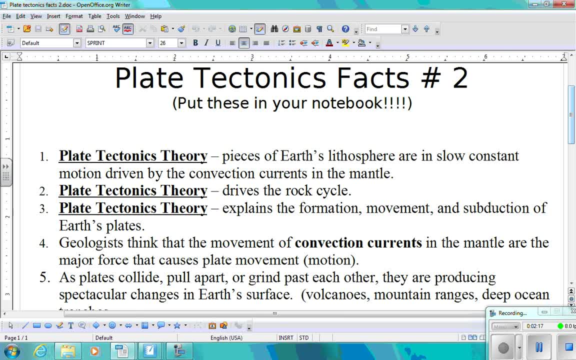 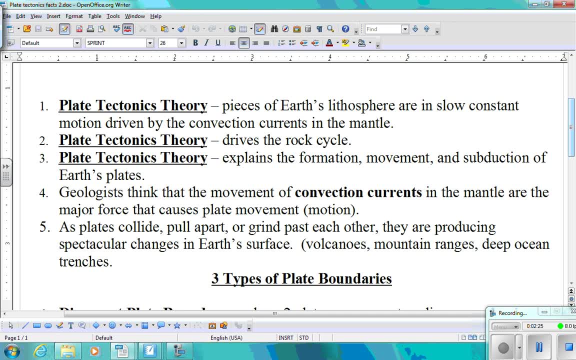 and now geologists know and understand this. with today's technology number five, as plates pull apart or grind past each other, they are producing spectacular changes in earth's surfaces, such as creating and making volcanoes, volcanoes erupting mountain ranges, deep ocean trenches and mid-ocean ridges. and 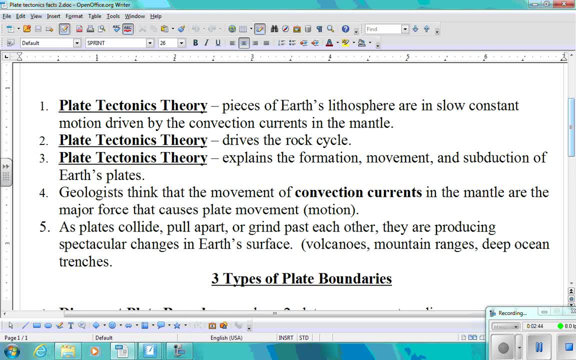 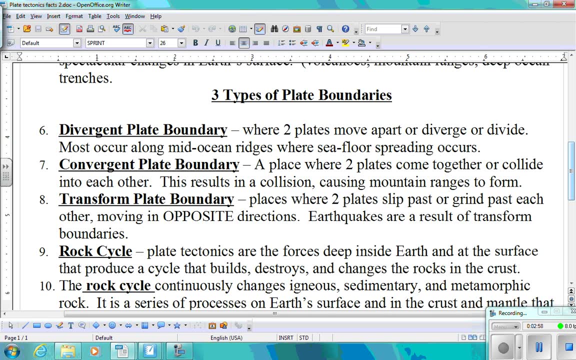 earthquakes occurring and the changing of rocks from igneous to sedimentary, to metamorphic- all of those things are happening because our plates are moving. the three types of plate boundaries that we need to know about: divergent plate boundary: this is where two plates move apart or diverge or divide- divide most. 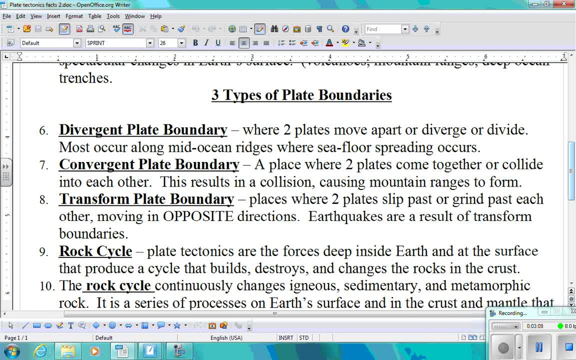 occur along mid-ocean ridges, and this is where sea floor spreading is occurring, which we will discuss it a little bit later today. convergent plate boundary: a place where two plates come together or collide into each other. this results in a collision, causing mountain ranges to form. number eight: transform. 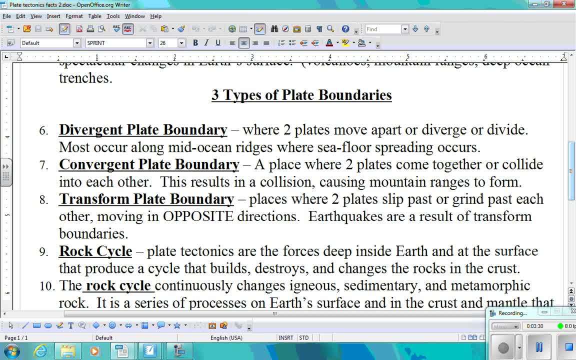 plate boundary. this is where two plates are going to slip past or grind past each other. they're moving in an opposite direction and often you'll find that earthquakes are results where we're transformed, boundaries are shifting and moving rock cycle. because of all this movement, the rock cycle occurs. plate tectonics are the forces deep. 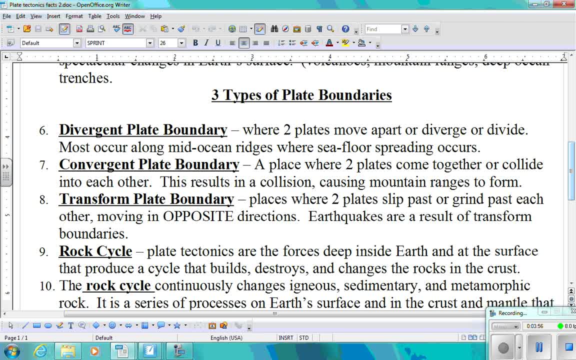 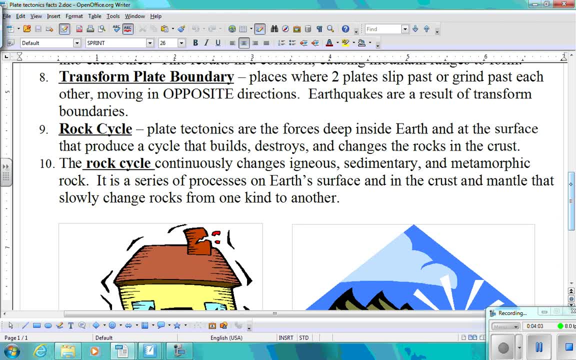 inside earth and that at the surface that produce a cycle that builds, destroys and changes rocks. in the crust, the rock cycle continuously changes igneous, sedimentary and metamorphic rock. it is a series of processes in the earth's surface and in the crust and mantle that slowly change rocks from one kind to 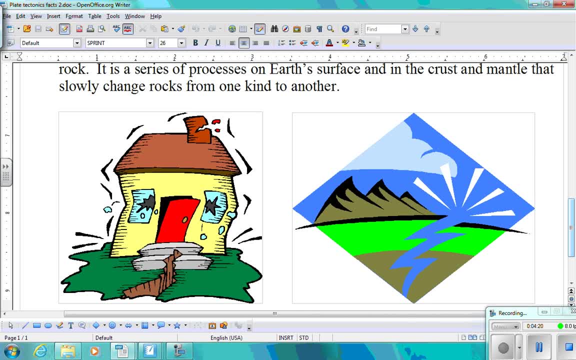 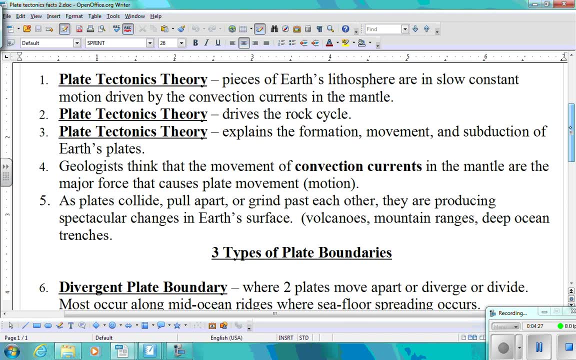 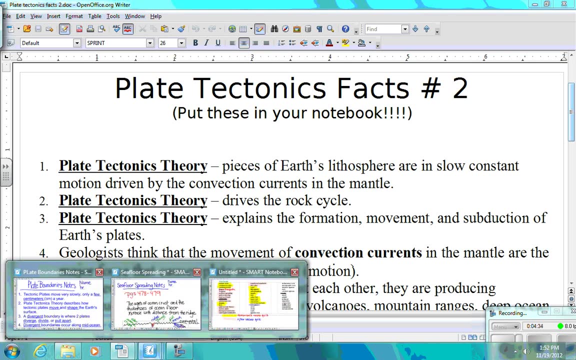 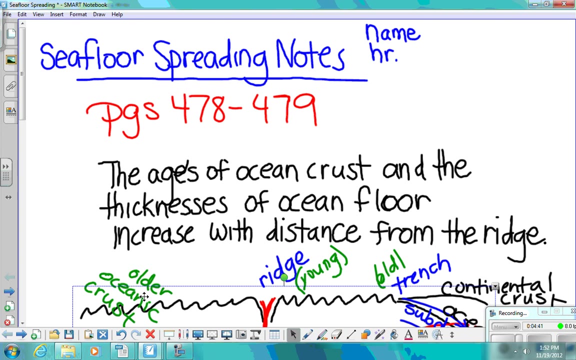 another. okay, so those are the notes you should have in your book, in your notebook now. all right, do you want to talk a bit about sea floor spreading? and you're reading. tonight you will be reading about sea floor spreading and it is a discussed on page 478 through 475 or, I'm sorry, 479. basically, sea floor spreading. 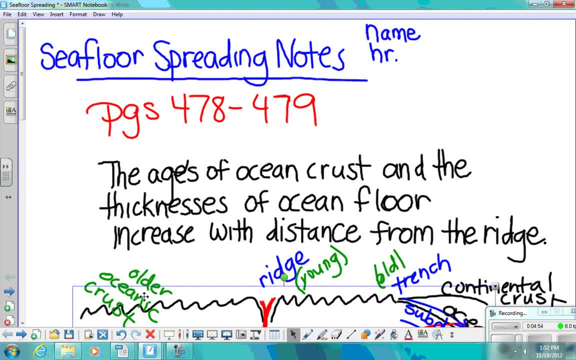 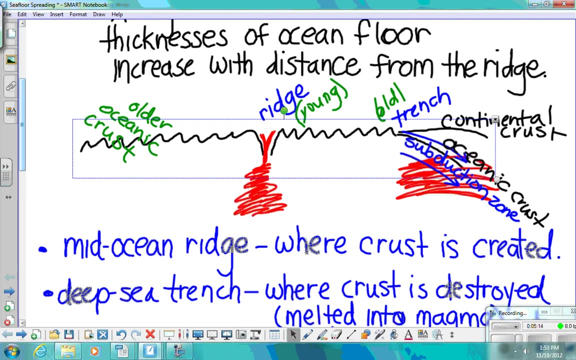 is telling us how or what the ages of ocean crust is and the thickness of the ocean floor, how that increases as the the ocean floor spreads apart and moves away from the mid-ocean ridge. so copy these notes into your notebook. I have an illustration here, too, that I'd like you to draw. here we have magma and 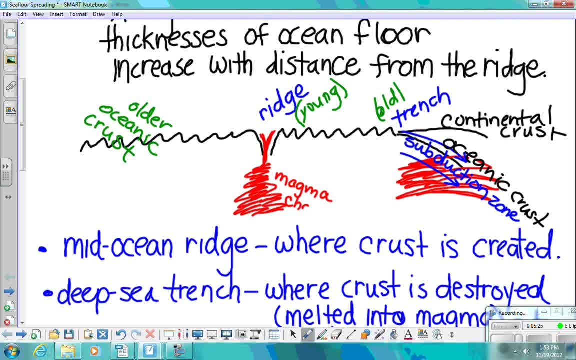 it's usually stored in what we call a magma chamber. but as sea floor spreads apart, right, there's a divergent boundary here. you can see it's a divergent boundary. it's pushing the sea floor in opposite directions. it's pulling it apart. as it pulls apart, that magma moves upward and 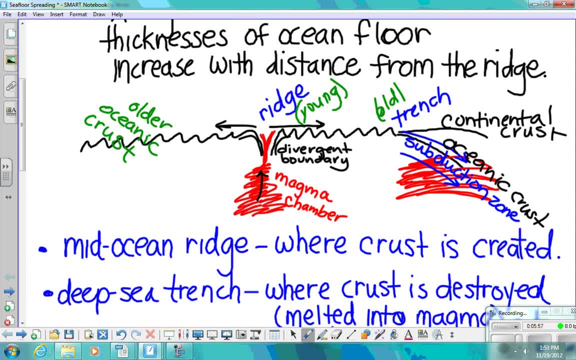 seeps out and it cools and hardens as the sea floor starts to spread it in each direction. so it's moving in this direction. okay, this becomes the older crust as you move further away from the ridge. the younger crust is right here at the, at the ridge. it's the newest. okay, so we're gonna add the word newest here, and 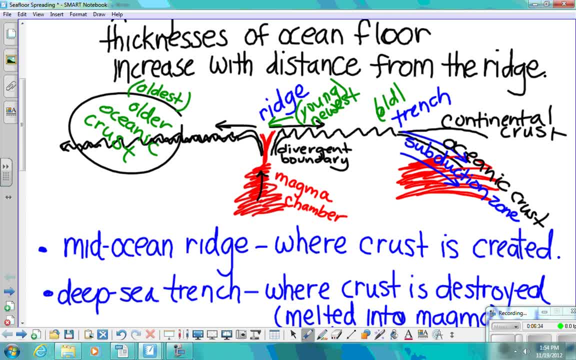 that oldest crust would be further away, so at the edge of the ocean, where it meets the continents, the land that we're talking about, the trenches here. okay, at the trench we have a subduction zone, so that means that part of this- sorry, I'm gonna move my red arrow back up- here- at the subduction zone we are. 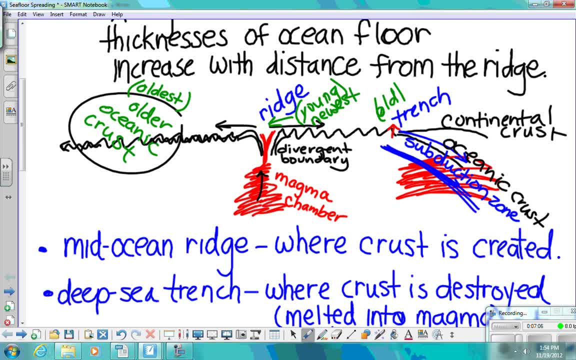 seeing this area. here we're seeing that some of this crust is being sunk downward- okay, so oceanic crust, because it's more dense, is going to sink when it comes in collision with continental crust. so we have our continental crust here, okay, and our oceanic crust down here, and the oceanic crust is going to sink and as it. 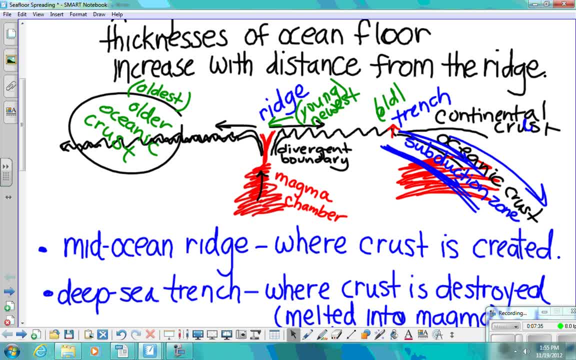 sinks, it's being pushed to lower layers of the earth and it's going to hit the mantle and it's going to melt. so we have two facts down here that we need to add to our notes. is that at the mid-ocean ridge, which is right here, okay, mid-ocean? 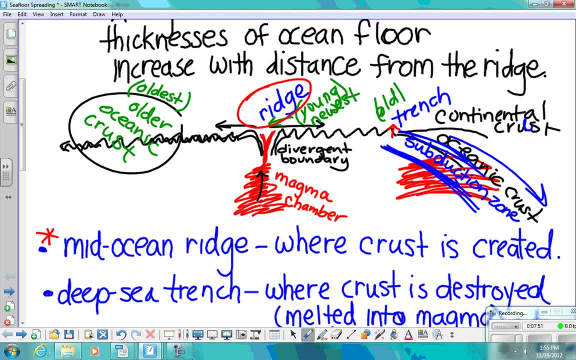 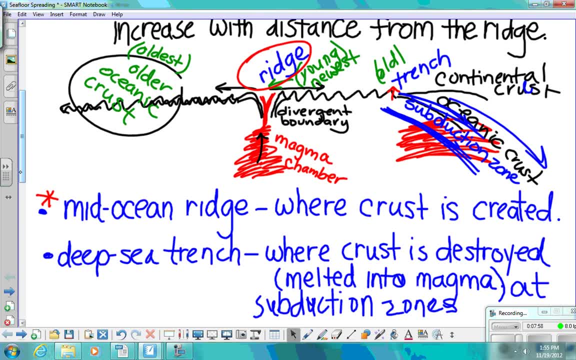 ridge is where crust is created. that's where the newest ocean crust is, at the deep sea trench. however, this is where oceanic crust is being changed or destroyed back into magma. okay, and that's called a subduction zone, and that's that area up here, okay. 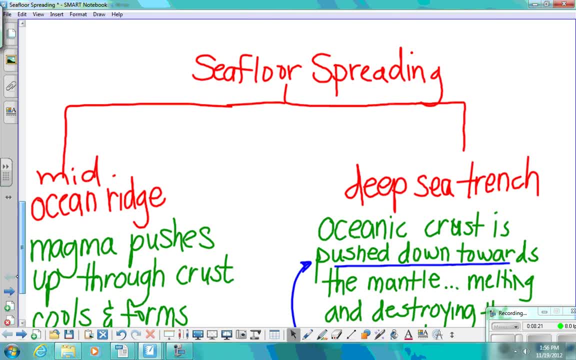 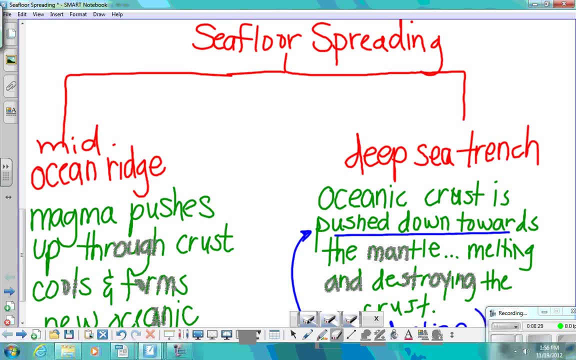 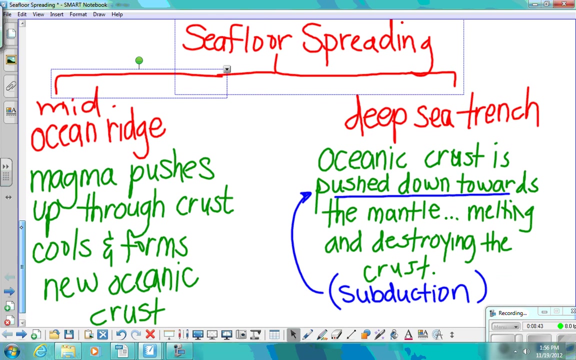 next, I want to talk to you about just breaking this down into a thinking map. okay, seafloor spreading- and let me just change this here real quick, I'm gonna make this a little easier for us to see all of it in one chunk. okay, that works. so seafloor spreading is the name of this tree map. we have two.